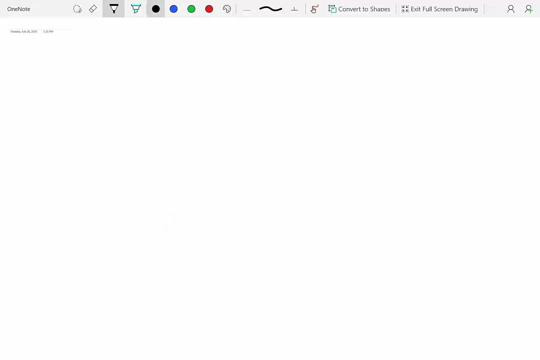 frame to use. so let's write that down. general method for solving planar rigid body motion problems and step one now. so this general method would essentially supersede the method that I gave to you before. so the method that I'm going to write right now will apply for the previous kinds of problems as well. 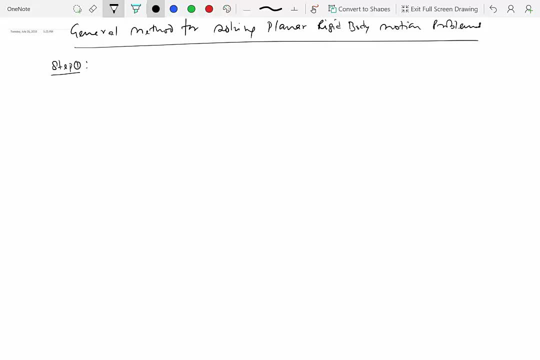 whether you use a translating reference frame. so step one is to decide between translating versus rotating frame. so for that, I'm going to give you a test. okay, simple test is to see if there is sliding happening over a rotating body. now pay attention to this. this is saying sliding happening over a rotating body. 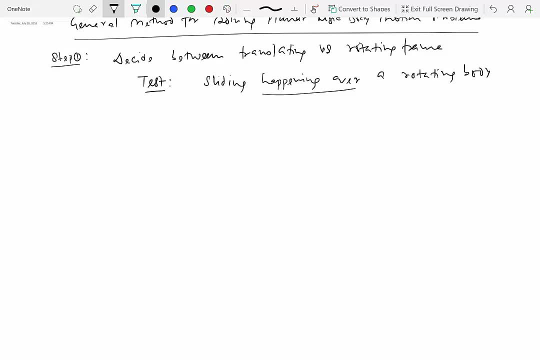 so, which means that if you pick a rigid body in the system that is given to you, on that politically rotating body, there should be some sort of sliding or relative motion occurring, okay. so let me give you an example. so this is an example. let's say I have an actuator, okay, and it's connected to a rotating body, like that. 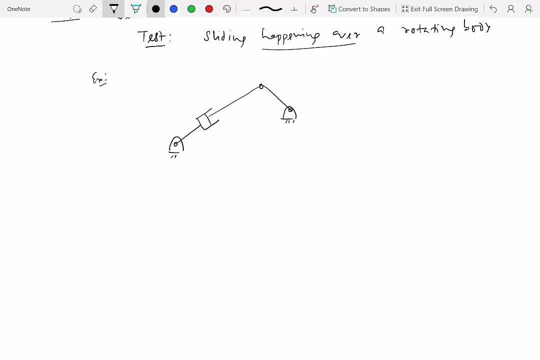 right, so this is the hinge, this is a hinge, this is a hinge and this is a slider, so which means that this slide is really allowed to this particular piston or slider is allowed to move back and forth as this rotates. okay, so which means that, essentially, the distance between the two of them is the distance. 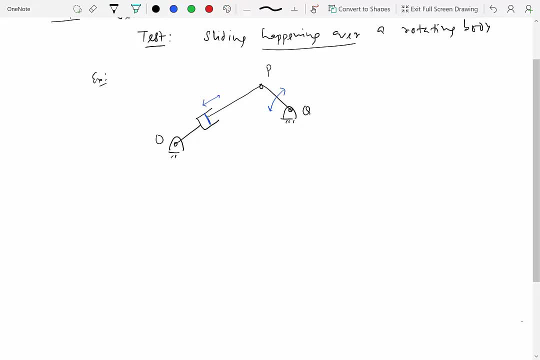 between. let's say, this point is O, this point is P, this point is Q. distance between O and P is changing. okay, so would this call for use of a rotating reference frame or a translating reference frame? this would call for a rotating reference frame because you have a rigid body OP over here which is 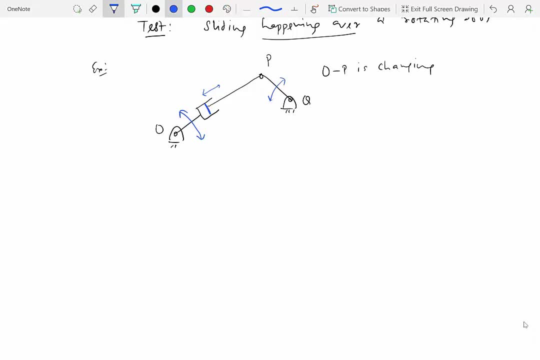 rotating and on this rotating rigid body that is sliding, happening. this slide, this piston is sliding on this rotating rigid body. another way of looking at this is to see that the distance between the two points on the rigid bodies between which there is a relative motion is going to be changing. 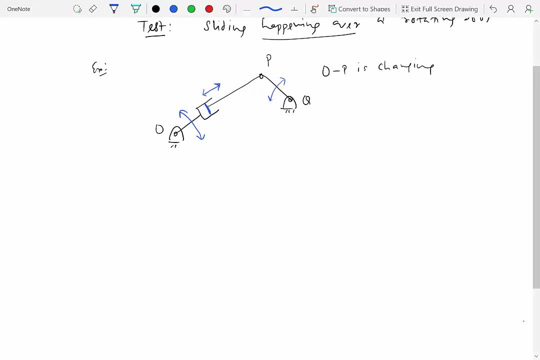 and you want to relate the velocity of those two points. so, for example, if I want to relate the velocity of the point O with the velocity of the point P, then the distance between O and P is actually changing. this R is changing. that doesn't happen for a rigid body where you are trying to relate the velocity in. 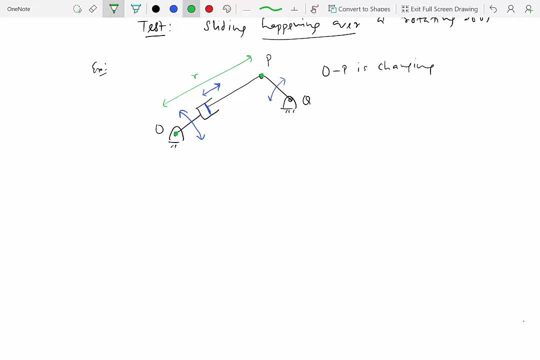 acceleration between the two points because by definition the distance between the two points on a rigid body does not change. but here now you're trying to relate the motion, you're trying to relate the velocity in acceleration of the two points on two separate rigid bodies, but there is a relative motion between the two another. 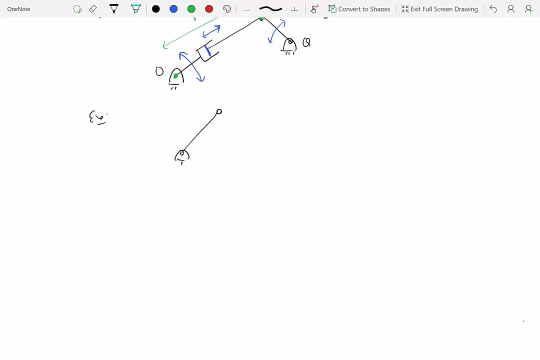 example. so this is a situation where we have a crank and we have a connecting rod and the piston is allowed to slide in this direction, right. so would this call for a rotating reference frame? do we have sliding happening on a rotating rigid body? yes, we do have sliding. 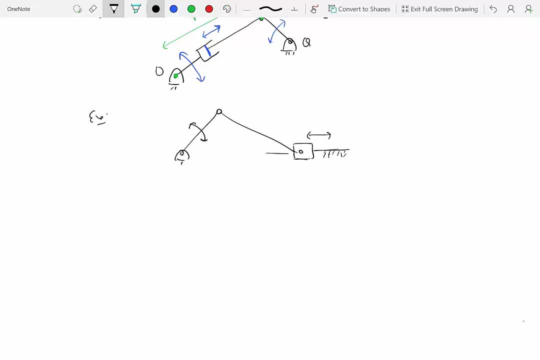 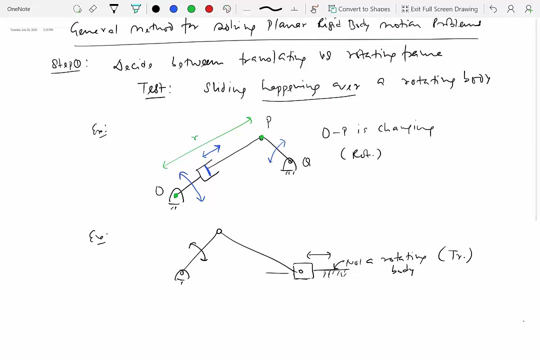 happening, but this sliding is happening on a fixed length. this is not a rotating rigid body. so this is not a rotating body, which means that in this case, you should be using a translating frame and in this case, we should be using a rotating frame. so the test says that if there is sliding happening over a 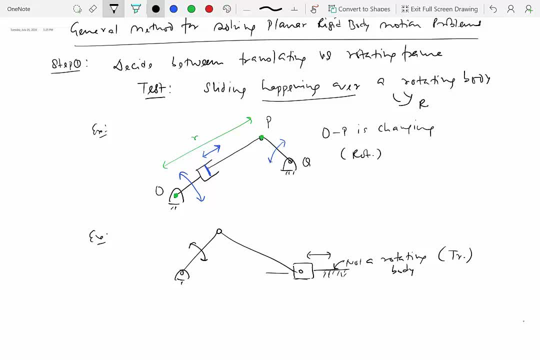 rotating rigid body, then use a rotating frame. so use rotating frames, otherwise you can use translating frame. then the next question is: okay, if this test is passed and we have to use a rotating frame, how should we show it? how should we align it? so one of the thumb rules is: you can, you can definitely. 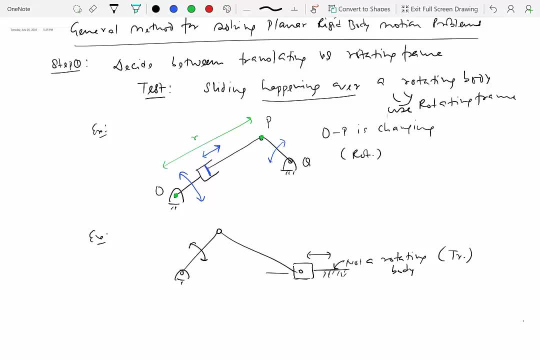 choose any version you want for showing the rotating reference frame, but one of the thumb rule says that you align your rotating frame with the rotating rigid body, primarily because in the rotating frame in that case writing relative velocity and relative acceleration expressions becomes simpler. so, for example, for the first problem over here, I will actually align my rotating 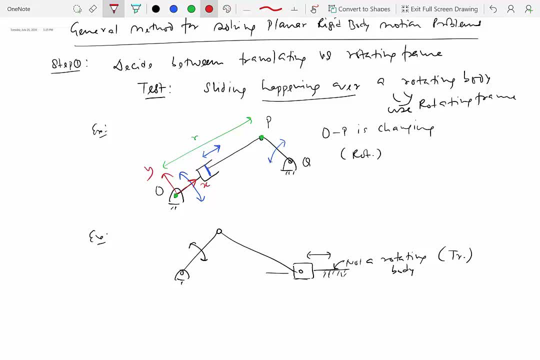 reference frame this way. okay, because in this reference frame, when I'm doing the analysis, when I write the relative velocity of the point P with respect to O, it will be along this direction. so V relative in this case, V relative in this case, would be simply V relative. I hat. on the other hand, if I 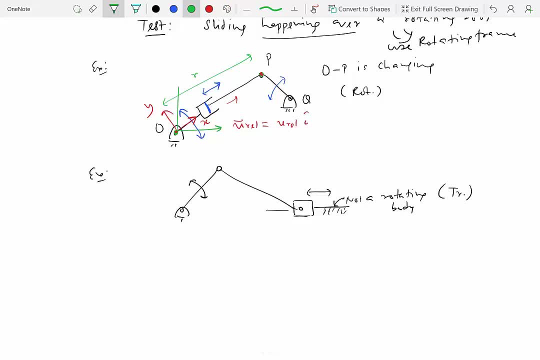 pick my rotating reference frame this way. if I showed it this way, then I would have to worry about what this angle is and I would have to resolve this relative velocity along these directions. okay, let me call it X prime, Y prime, all right, but then you have to keep in mind that once you show your reference frame, 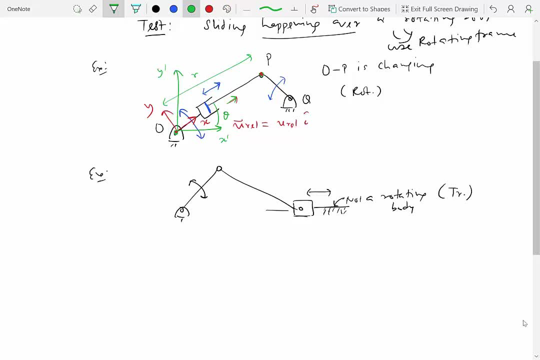 in one direction. so the red one is how I'm picking. then every vector, quantity, every position vector, every velocity, every acceleration has to be written with respect to that reference frame. in fact, that's one of the commonly made mistakes by the students, so I'm going to come back and repeat that point. 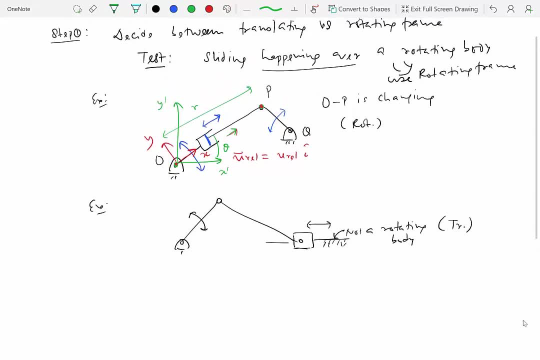 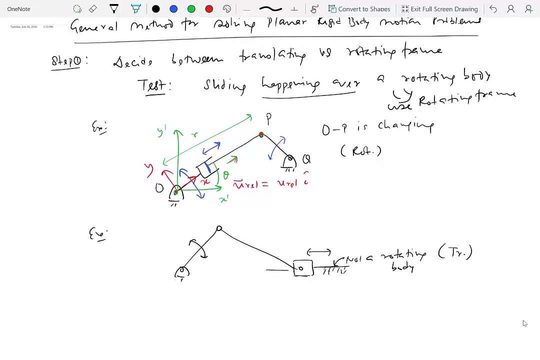 once again when I'm solving the problem. okay, so let's get back to our method. so the first step is to decide between translating versus the rotating frame, and the test for deciding between the two is to recognize that there is sliding happening over a rotating rigid body. now this test actually works most. 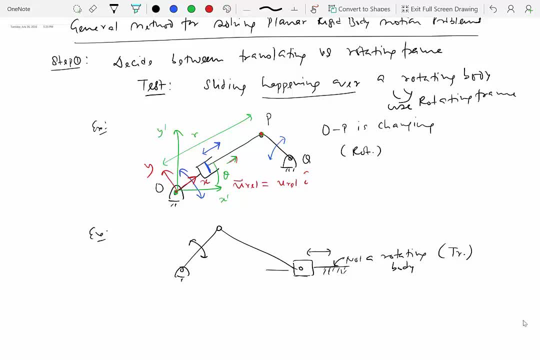 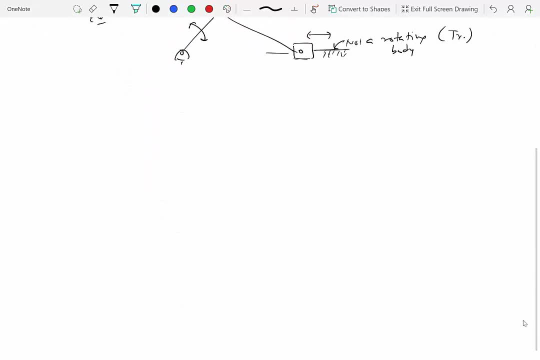 of the time. but there are some situations where you wouldn't see any sliding happening over a rotating rigid body. but you can still use- you know- the equations that we have derived before. so another example is: let's say, I have, you know, a merry-go-round right, so this can be seen. 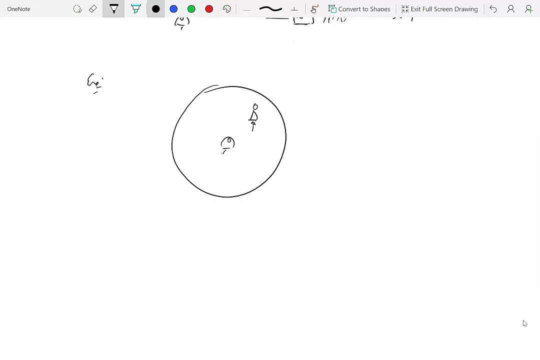 as a disc, and there is a person standing over here and this person is, you know, fixed with respect to the merry-go-round. so as this merry-go-round rotates, this person is also rotating and this merry-go-round is in a park and there is a walkway in the park and there is another person. 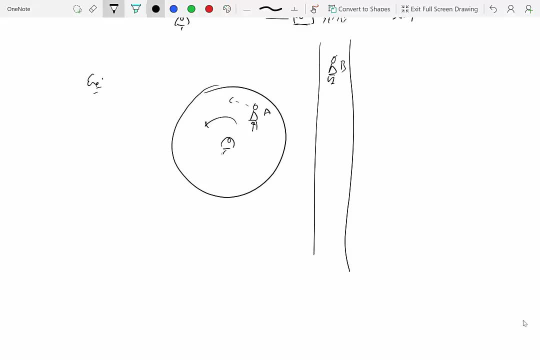 who's walking here. so let's call this person A and this person B, and this person is actually walking this way, right? so in a situation like this, if somebody said, can you tell me what is the velocity, relative velocity B as seen by A, it turns out, for problems like these, use of rotating reference frame. 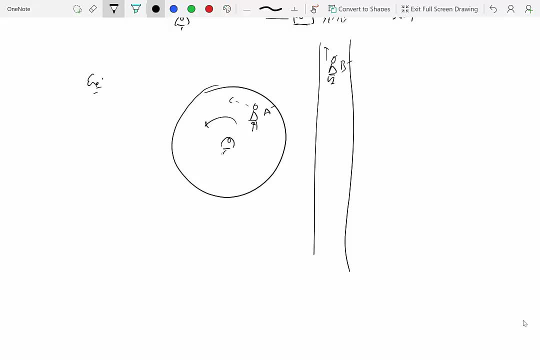 becomes important, because what you have over here is the reference frame. if you attach your reference frame to A, which is what you would have to do if you're looking for, let's say, a relative velocity B of B, so I'm looking for relative velocity of B as seen by A, and what is 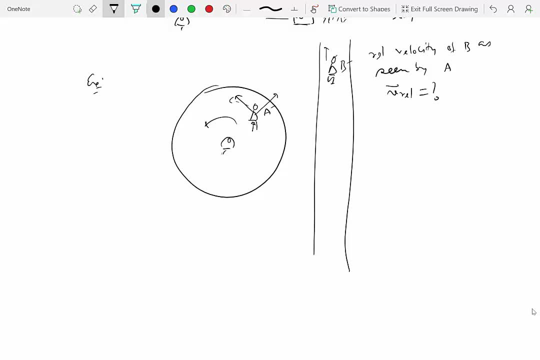 that quantity. that is basically V relative. so the question is: what is V relative? and if you try to use your previous knowledge of computing the relative velocity by saying this relative velocity is VB equal to VA plus V relative. in a sense, you are writing this as a velocity of B with a. this 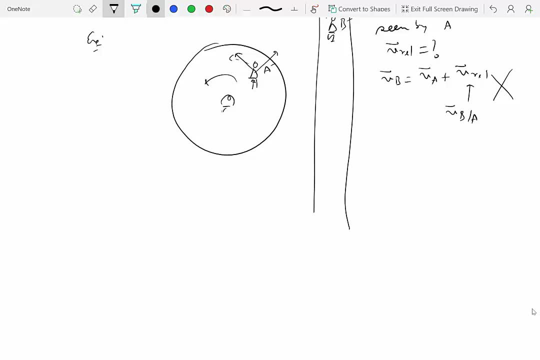 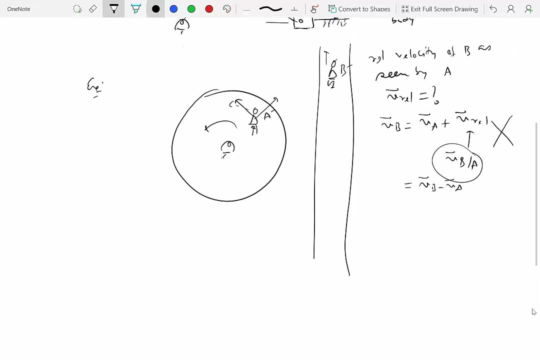 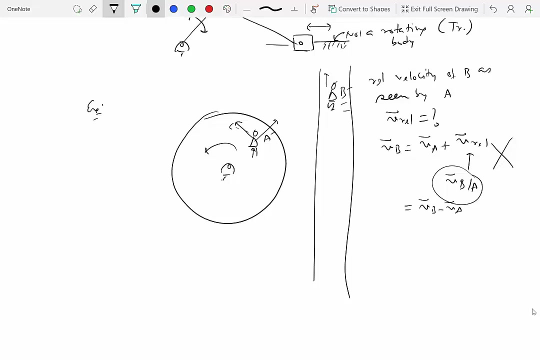 would be wrong, because the relative velocity in this case is actually not equal to VB over A, which is simply VB minus VA. so if you simply did the subtraction between the velocity of B and that may be given to you as seen by an inertial reference frame or a stationary observer. let's say this is my. 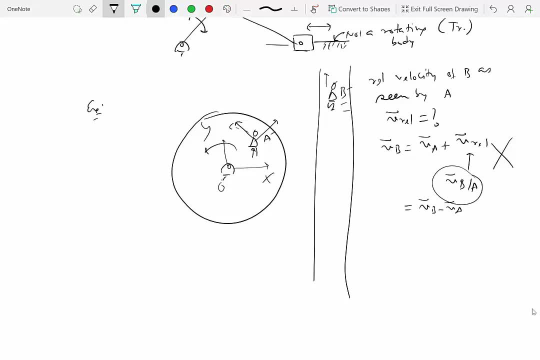 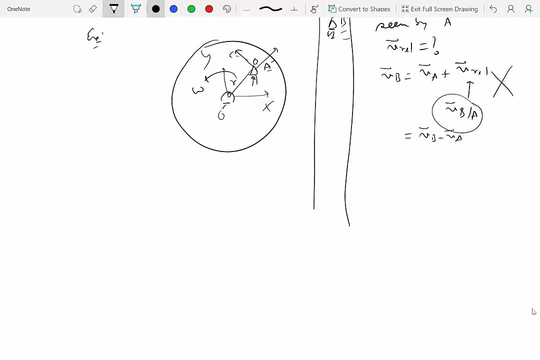 stationary or primary reference frame and you subtract with the velocity of A, which you could also determine because you know the angular velocity, you know the distance between the two, then you would be making a mistake, because that is not the velocity as seen by A. why this is? 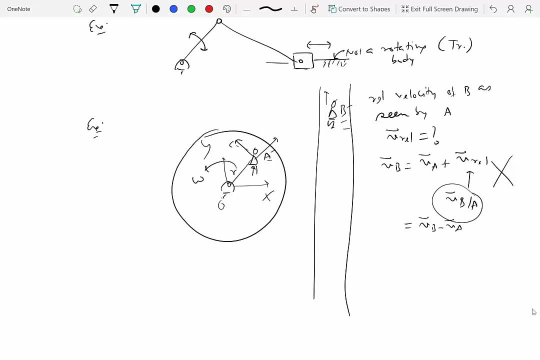 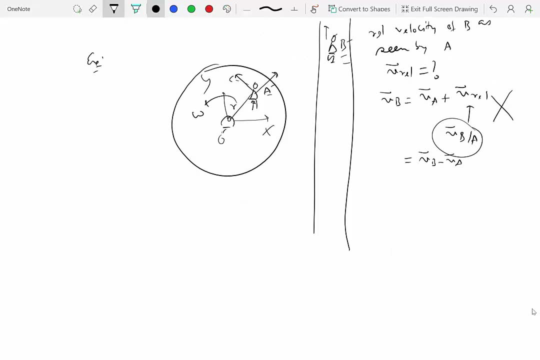 not correct. this is an important point that may surprise you if you're coming with, even with a strong physics background, because you have attached your reference frame to A, which is actually rotating with the disc, or the merry-go-round, this relationship where a velocity simply subtraction between the 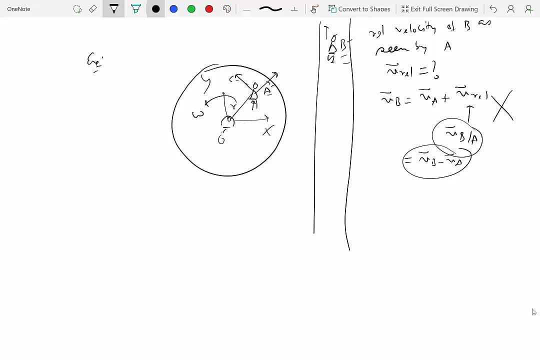 two velocity is valid only when you have a translating reference frame. so if you wanted to solve this problem, you would have to solve this problem by attaching a moving reference frame to A like this, and then you would have to use your equations which relate these two velocities in the following way: 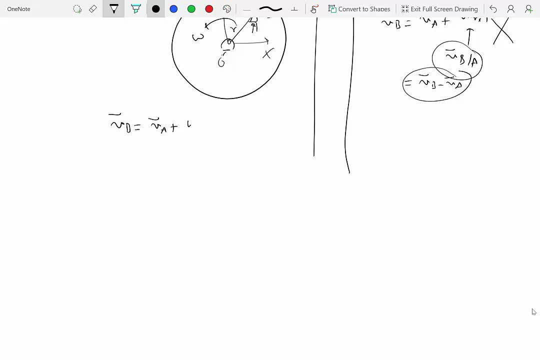 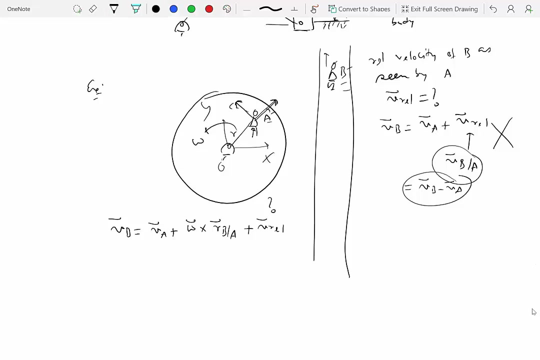 velocity of B equal to velocity of A plus Omega cross R of B with respect to A plus V relative, and it is this V relative that you are looking for now. in this case, if you look at this, we are using rotating frame equations and you can see that there is no sliding happening on a rotating rigid body at. 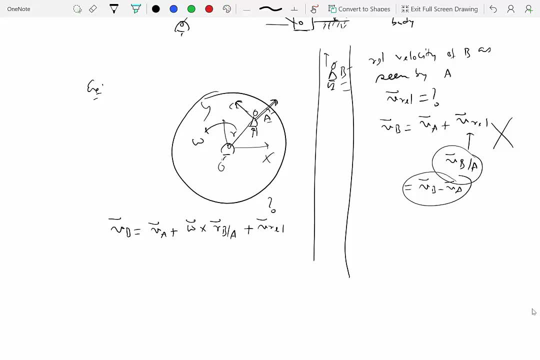 least not in the sense that we have understood it so far- right, because B is really not on A yet there is sliding happening in the sense that the distance between A and B is actually changing the distance. so as A rotates the B is maybe farther from A right. so if let's say A comes here and B is over here, the 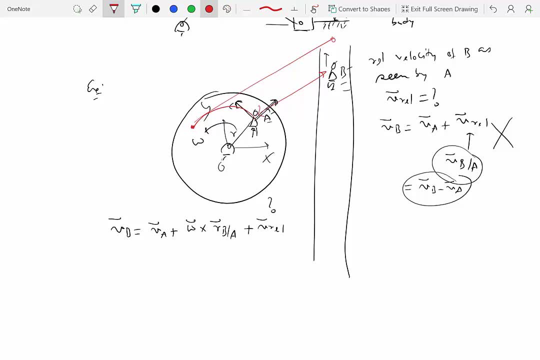 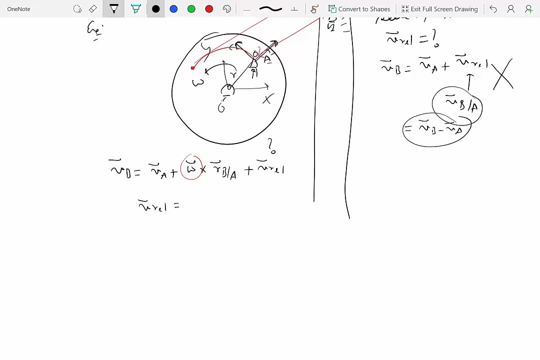 distance between A and B has changed right, so there is relative motion between B and A, and A itself is actually mounted on a rotating rigid body, and that's why you have this term as well. so in this particular case, if you were really interested in calculating the relative velocity, it would be VB minus VA minus. 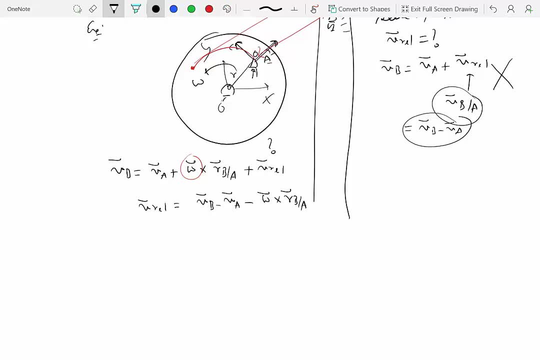 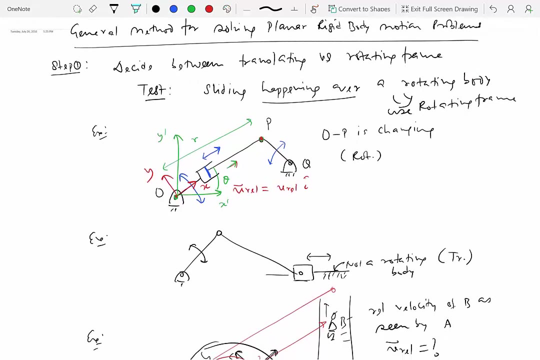 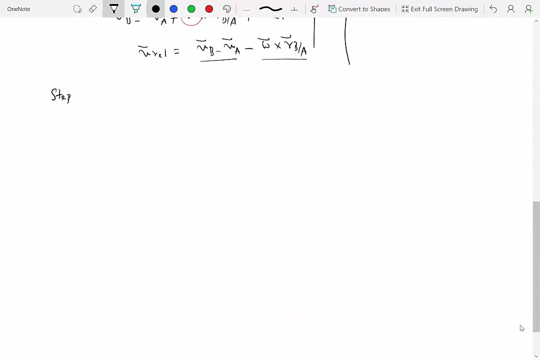 Omega cross R of B with respect to A, so you do subtract VB from VA, but then you also subtract the rotational term. okay, so step one was decided- what kind of reference frame to pick- translating versus rotating- and then step two is to show the frame. okay, so let's write that it's step two: show the. 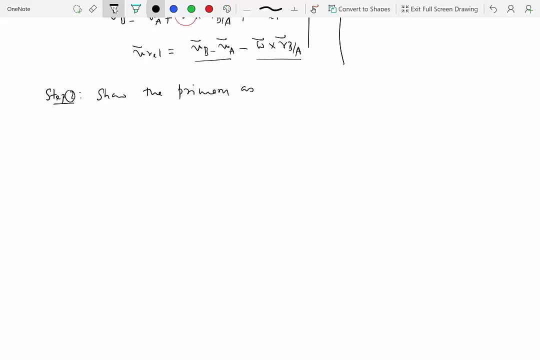 primary as well as moving reference frames and, as much as possible, you should align moving reference frame with rotating body. okay, so step three would be similar to what we did before, which is to identify the motions of various rigid bodies. so actually, from this point onward, the method is same as.